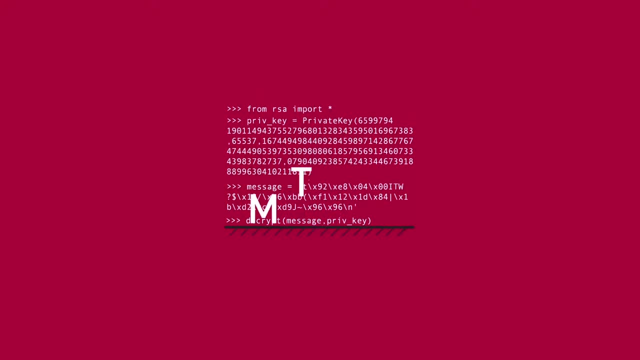 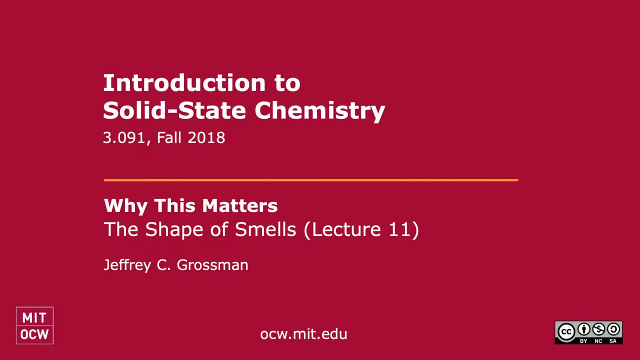 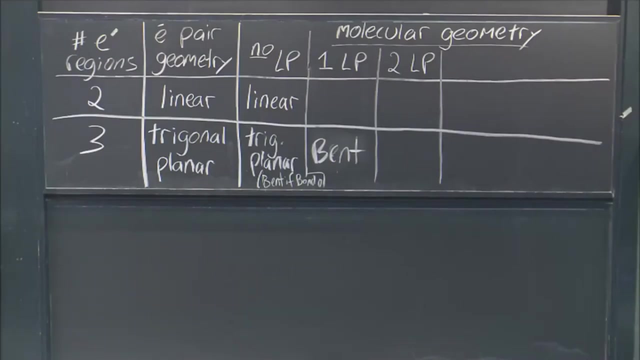 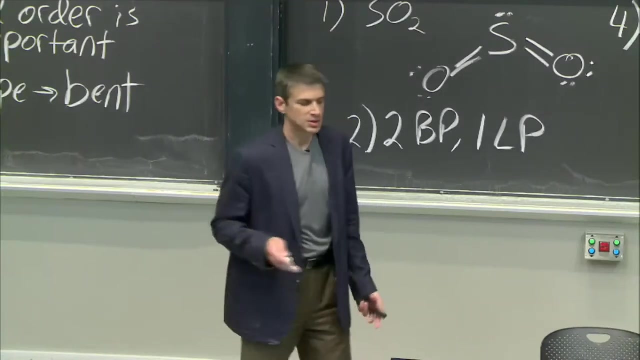 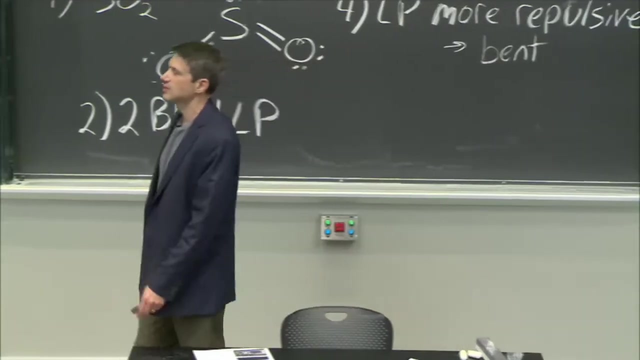 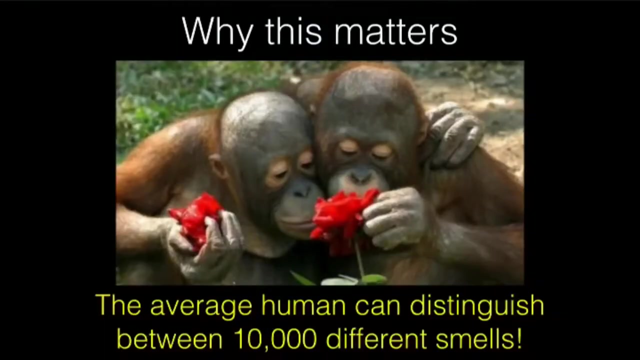 Why does shape matter? I told you shape mattered in the very beginning. but why does it matter? Isn't it just important to know what the chemistry is, and not the actual shape? Why does the shape matter? And so I thought I would give you an example of that, with smell and yeah, right, exactly. 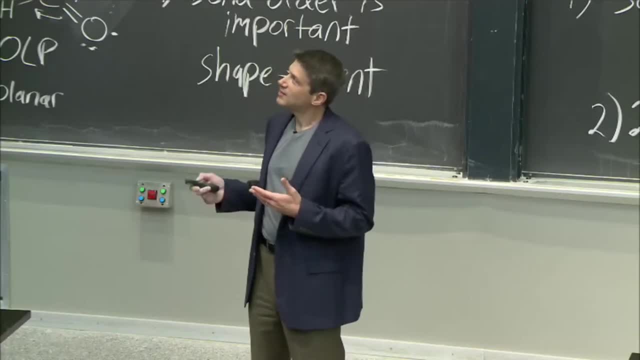 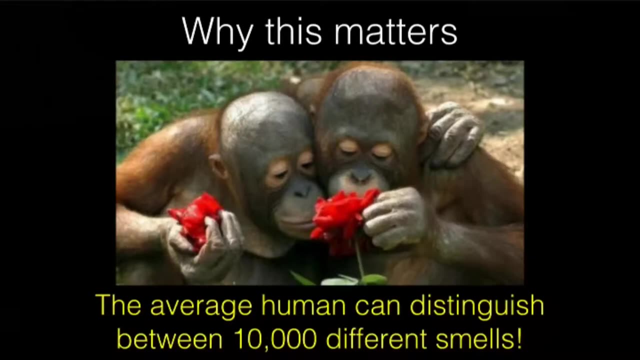 And I actually think we should do this more often. I feel like this is inspiring. We talk about stopping and smelling the flowers, but do we actually do it? And look at that, They've got one arm around the other. This is a moment. 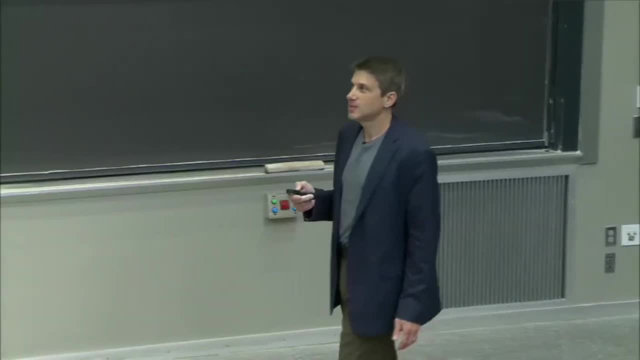 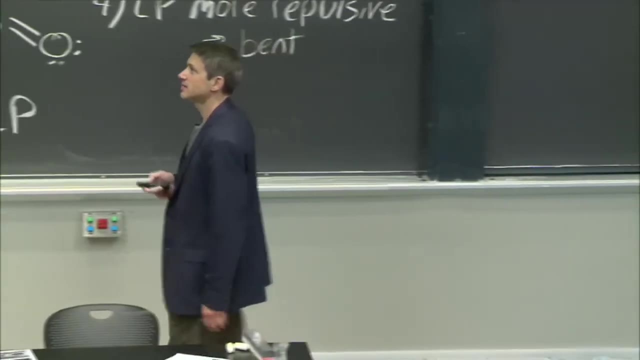 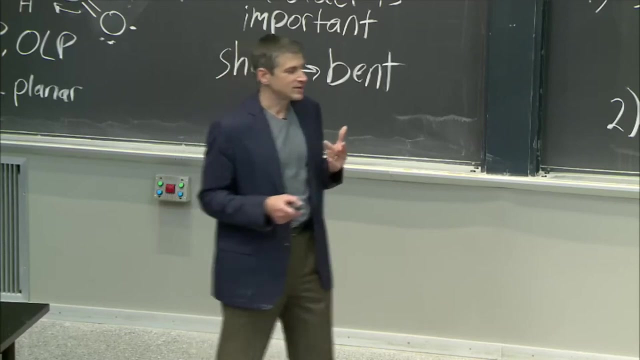 You can't share this moment on Instagram. You have to put your phone down and be there. You have to have this moment, and I highly encourage you to be inspired by this. Now, smell and taste are actually related, and smell is actually a fascinating thing. 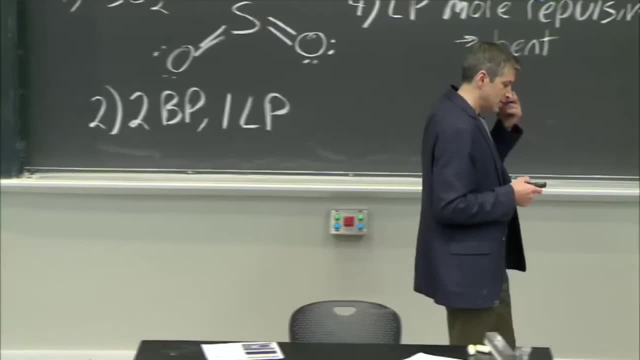 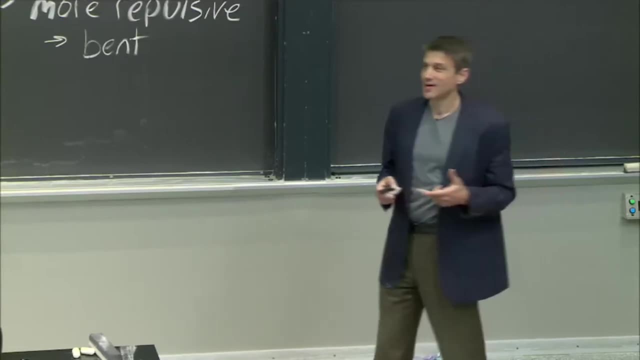 We can smell about 10,000 different smells. It's remarkable A dog can smell between 10 and 100,000 times more right. So if you do the analogy that people do with vision, we can see a third of a mile a dog. 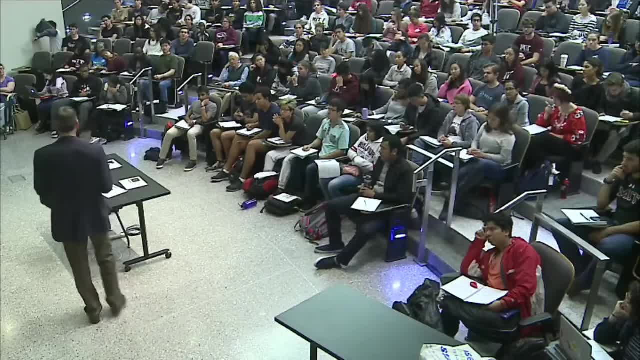 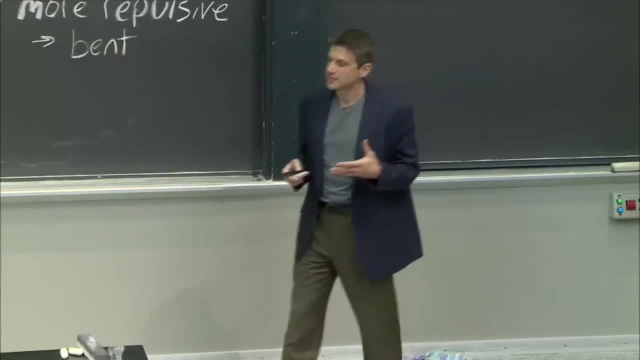 can see about 3,000 miles. right, That's pretty cool. But the question is: why do we smell? How do we smell, How do we taste? And it turns out that the way that we distinguish from one smell and one taste in another has 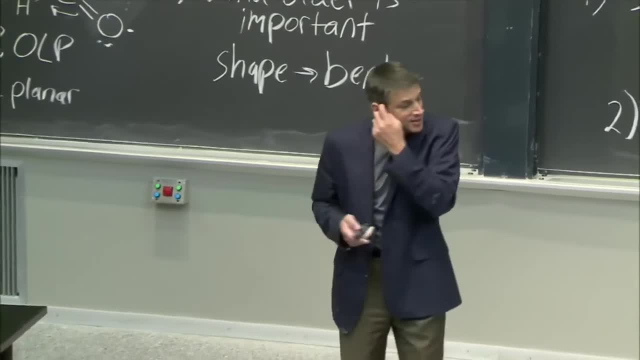 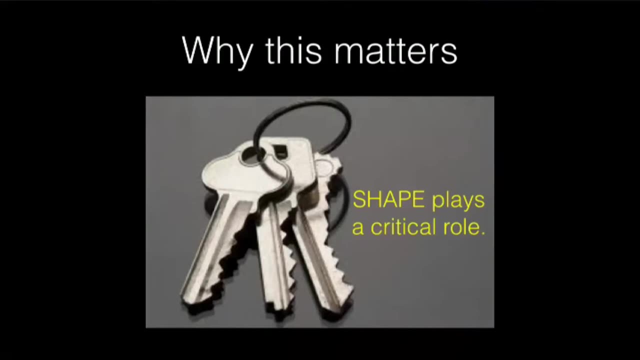 to do with the shape of the molecule, And so, just like a key right With a key, it's all the same material, It's the same chemistry in the key, but the shape is different. That can unlock the door or not. 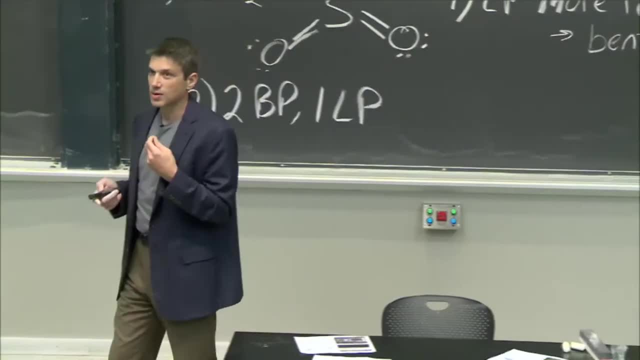 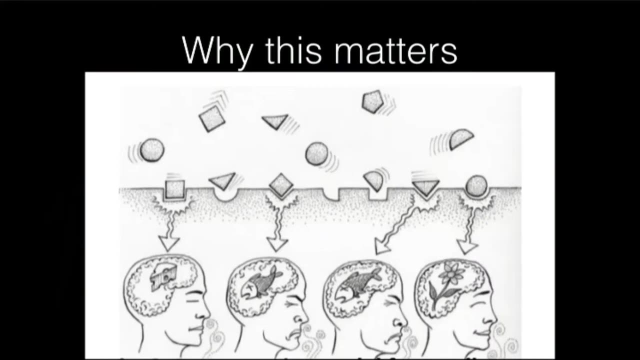 That is literally how our receptors work. Right, Our receptor cells work for taste and smell. This is a cartoon. I found that I kind of like: See, OK, shapes, circles, squares, right, OK, And some shapes come in and they make happiness, flowers and stuff. 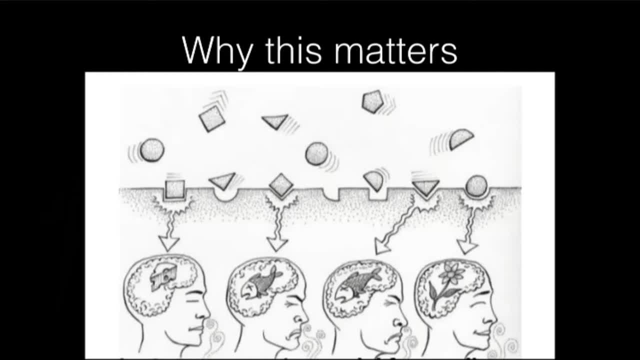 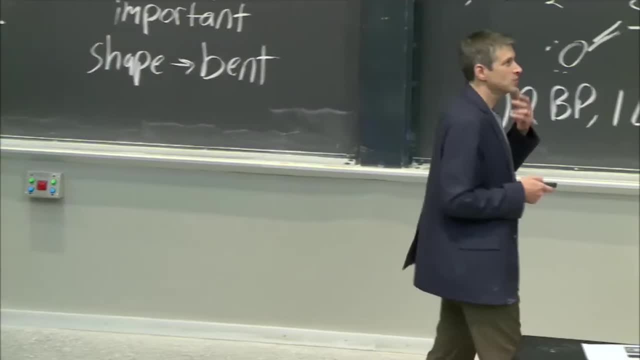 I don't know, Is cheese happy? It looks neutral. I would get happy with cheese. But anyway, fish for some reason. But you know it depends. But it's shape dependent. Now the thing is, taste works that way too. 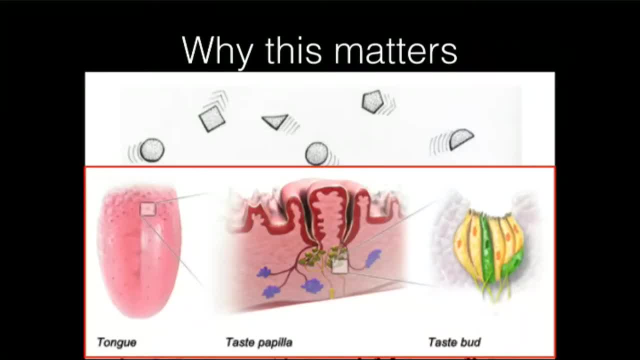 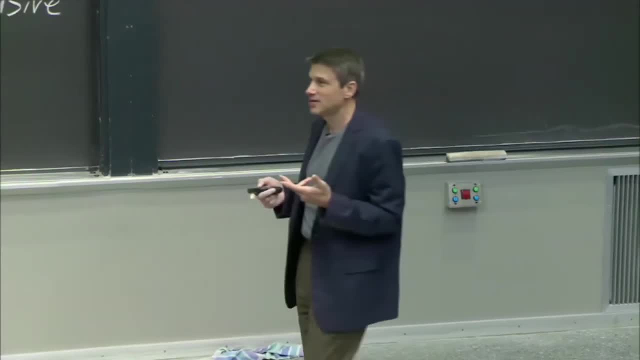 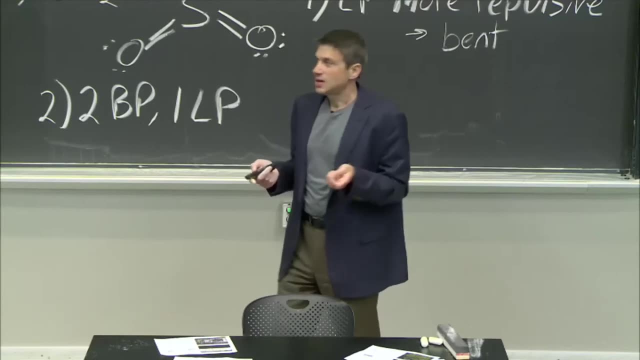 So this is what's happening in your tongue. You've got these taste buds. We've all heard the word taste bud, right, But what is really going on? What is really going on is a combination of chemistry and shape recognition. So the taste bud. if you look at the taste bud, 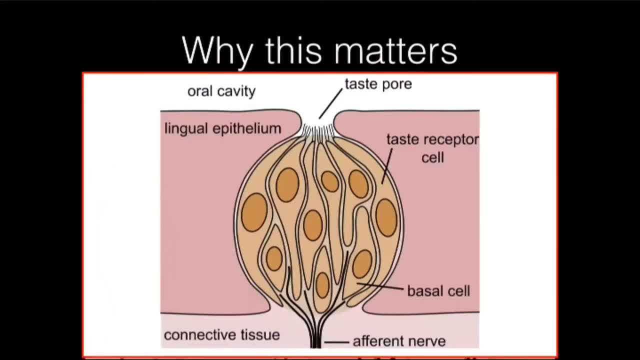 that's inside of these little pores inside your tongue. There's a blow up of it, And so this is what the surface of your tongue looks like, And there's a little pore And there's little filters in there that help certain molecules kind of get in there. 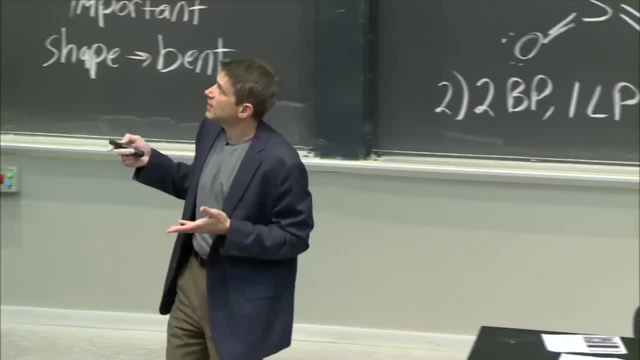 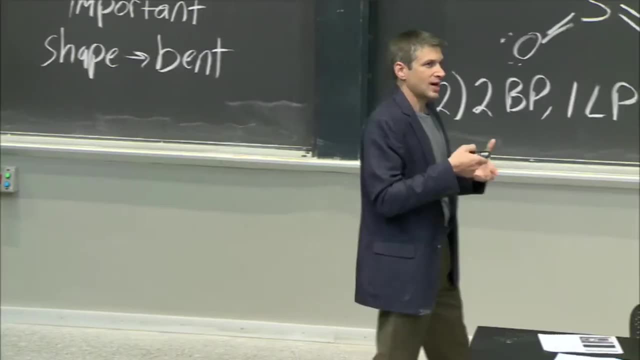 And what happens when they get in there? Well, what happens is you've got these taste receptor cells that are like lock key pairs. They actually only look at the circle or the diamond And they can tell you which one is which, And that's a major part of how we distinguish. 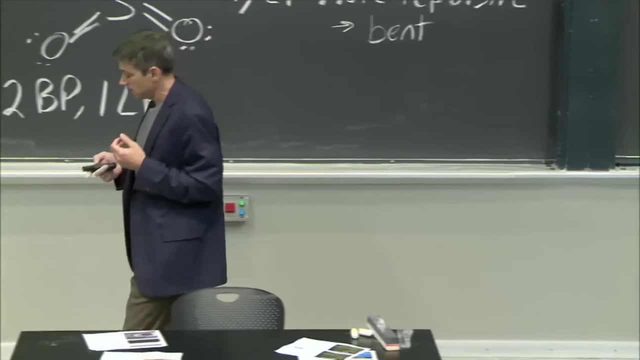 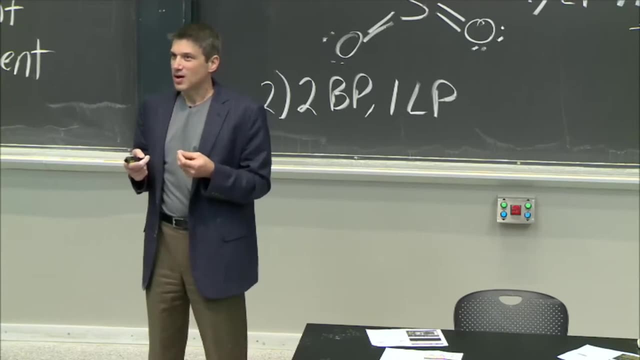 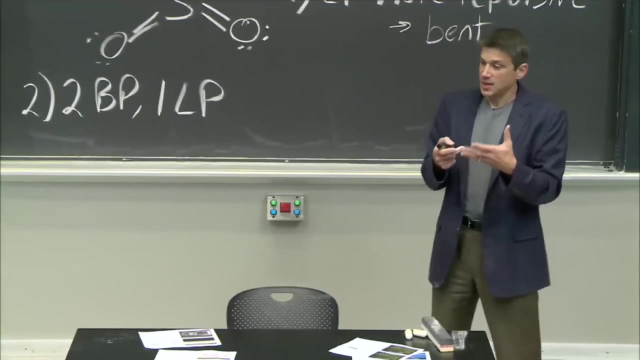 from one shape to another, And it's actually so. it goes back a long way. Why? Because shape and smell are literally survival. They're literally like: if you taste something and it tastes poisonous, don't eat it. You live right. 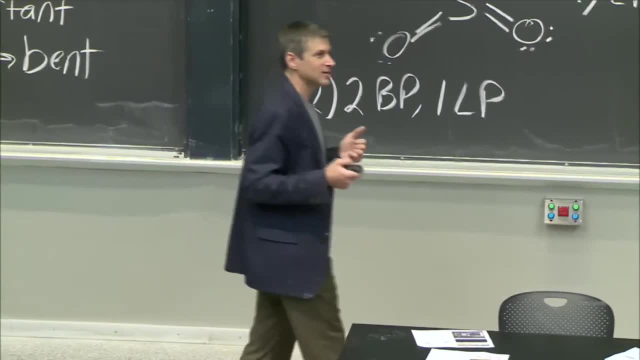 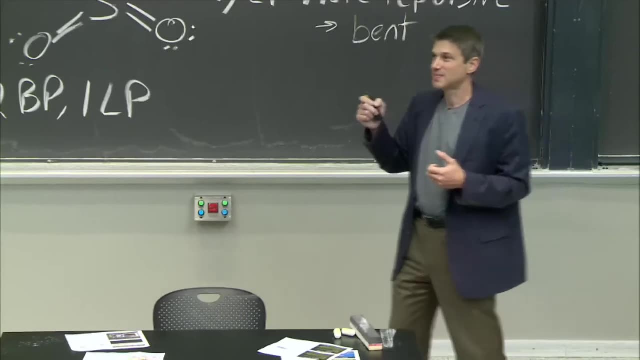 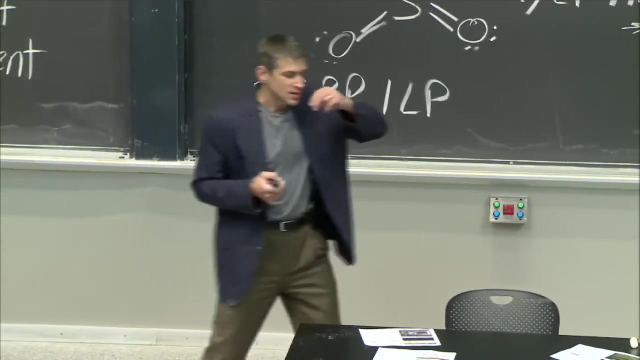 So it is a very emotional thing to smell and taste because it is actually coupled to your very survival. And Democritus himself- Democritus, our friend Democritus- said that shape must be involved. He thought that because things that taste bitter are sharp. 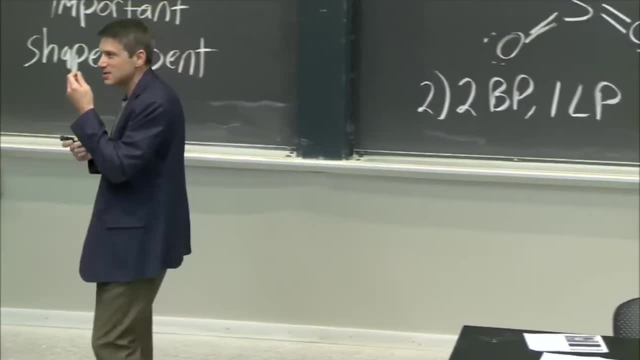 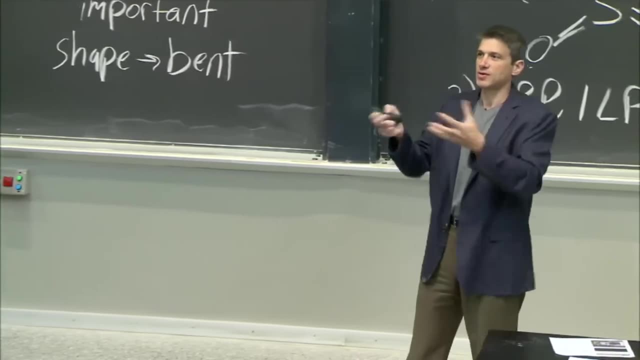 that the bitter molecules were sharp. They must have sharpness to them, like shards of glass, That's how he imagined it. And the sweet molecules were sort of these soft, fluffy spheres That's not that far off from being sort of what. 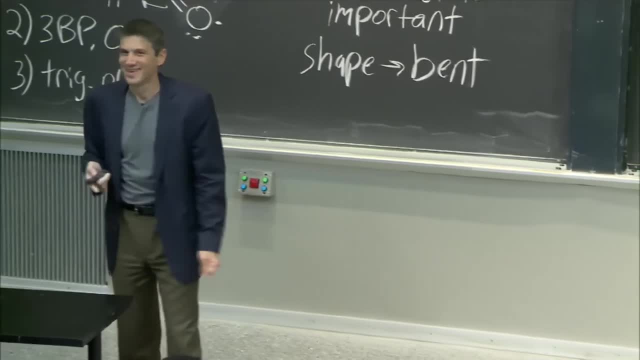 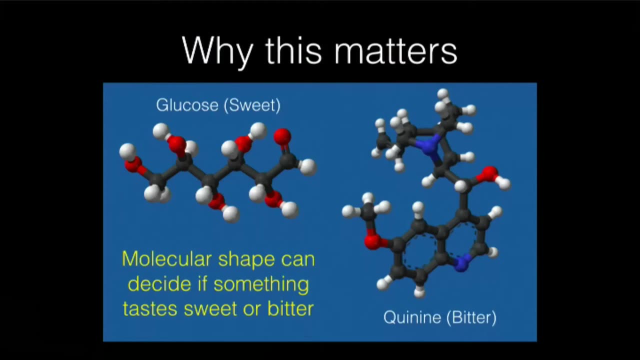 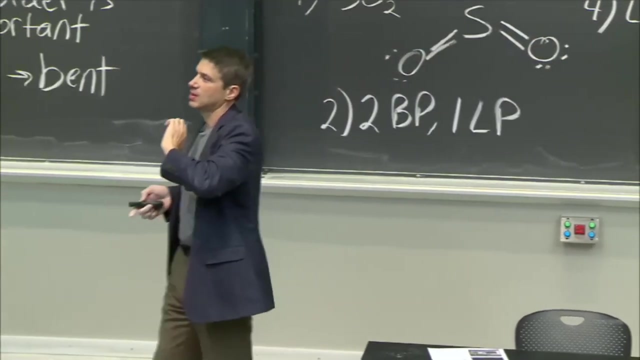 happens a little bit. But when we look at glucose and quinine we say, OK, those are very different chemistries, So it might not be It is obvious why one of them tastes so different than the other. But check out this example. 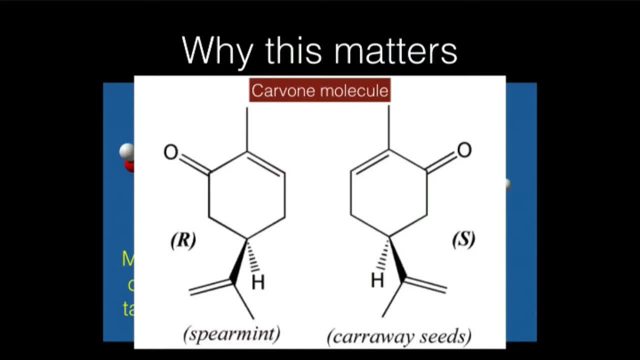 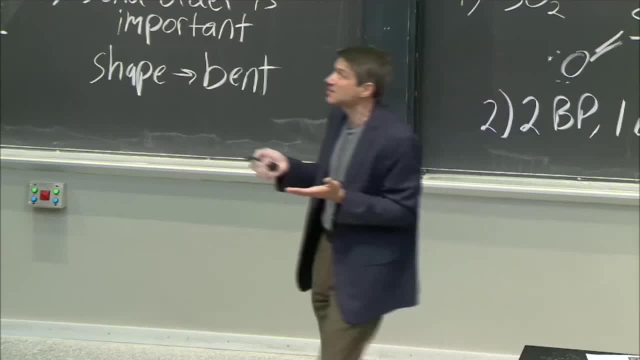 This is the same molecule, the carbonic molecule, that is called an enantiomer, which means that it has handedness. It's the exact same chemical formula and the exact same structure, except for one is like this and one is like that.